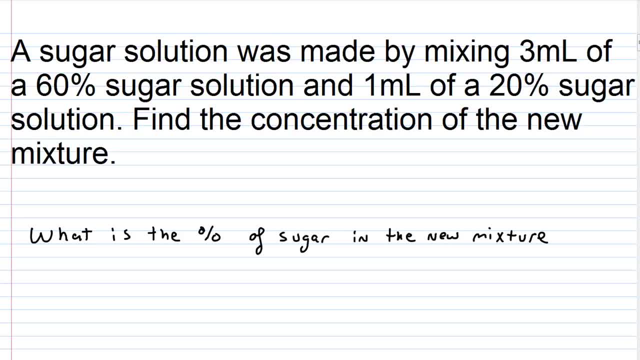 looking for. So how are we going to find this percentage of sugar in the new mixture? Well, what we need to do is take the total amount of sugar in milliliters in the new mixture and divide this amount- the total amount of sugar in milliliters in the new mixture- and divide. 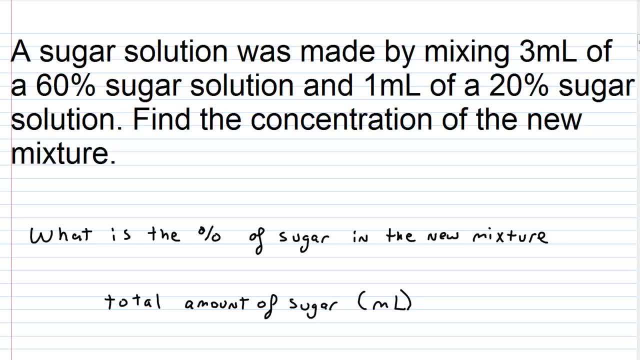 this amount by the total mixture itself. So I'm going to divide this amount by the total amount of sugar in the new mixture. So I'm going to divide this amount by the total mixture. Okay, and everything here is measured in milliliters. All right, so if we want to know the first part here, the 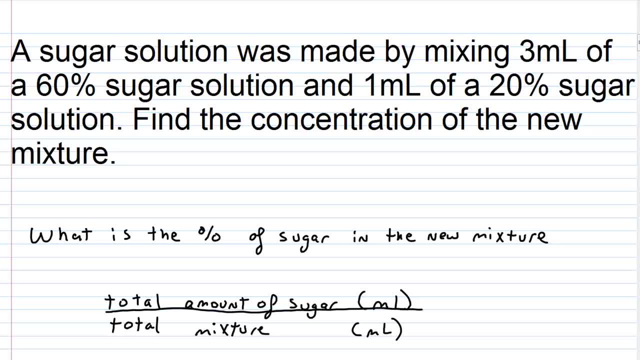 total amount of sugar in the new mixture. I can just go up here and re-read back to the problem. I'm told that what we put in the new mixture was three milliliter solution. that contains a total amount of sugar. So I'm going to go up here and re-read back to. 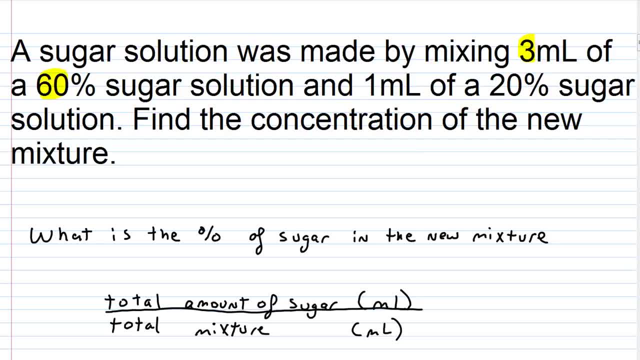 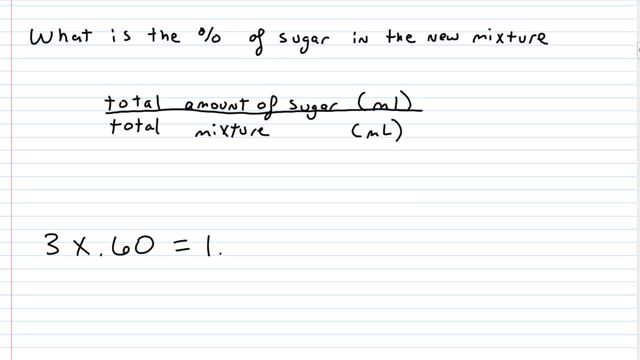 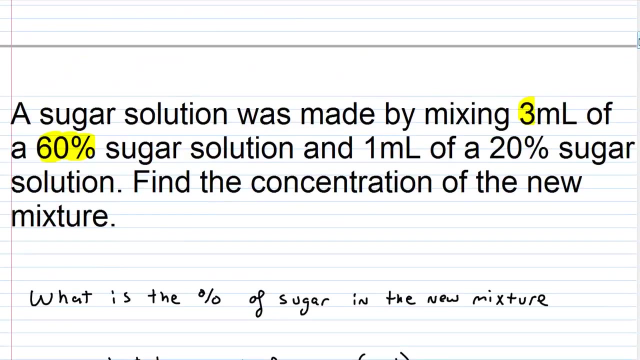 what we put in the new mixture. I'm told that what we put in the new mixture is- and never gets Photo into her- Perfect. so that's going to give us 1.8.. So this would be the amount of sugar that's in that 3 milliliter solution. That's the amount of sugar in this part. Then for 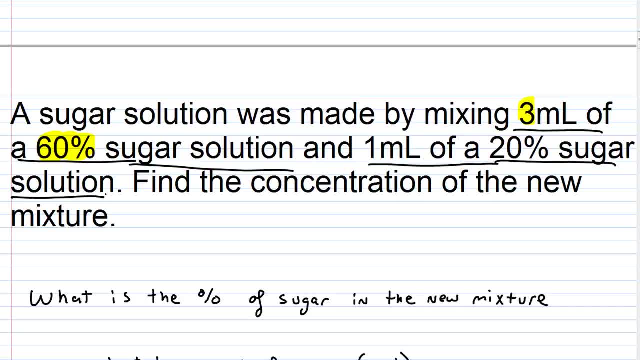 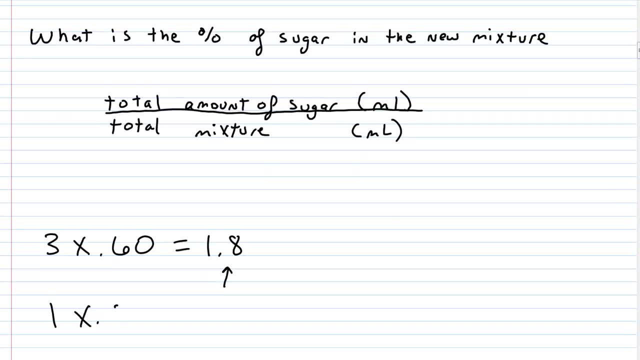 this part. I'm going to multiply by 3, by 2 упq0. little by little will result one milliliter of a 20% sugar solution. I'd multiply 1 times 0.20 and of course that's 0.20.. So 1 times 0.20 is 0.20.. So if I take these two amounts here and I 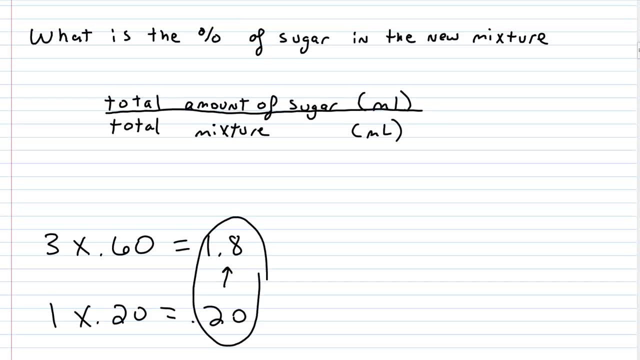 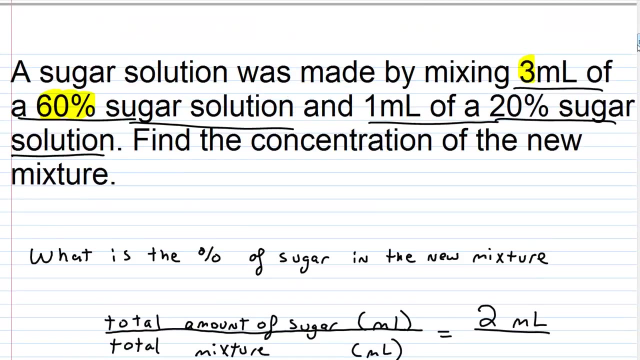 add them together, I'm gonna get the total amount of sugar that's in that new mixture. Okay, 0.20 plus 1.8 is 2.. Okay, and then the total mixture itself is really easy to figure out, because, if we look here again, the solution was made by. 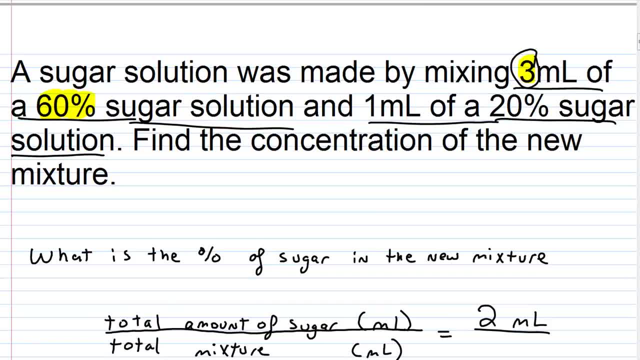 mixing 3 milliliters of a 60% sugar solution and 1 milliliter of a 20% sugar solution, So that the new solution, the total amount of milliliters, would be 3 plus 1, that's 4.. 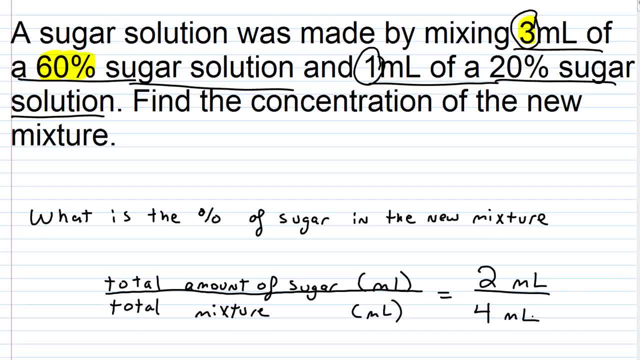 So this down here is 4 milliliters. okay, Now let me just run back through that one more time. The top part is the total amount of sugar in milliliters in the new mixture. I got that by taking 60% of the 3 milliliters here. 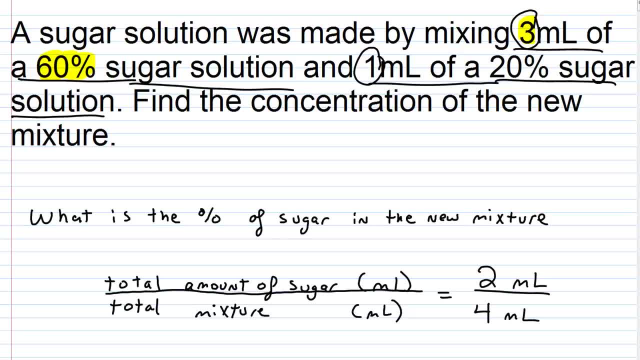 60% of 3 is 1.8. So I got that plus I took 20% of this 1 milliliter here That's going to be 0.2.. We had 1.8 and 2 together and we get 2.. 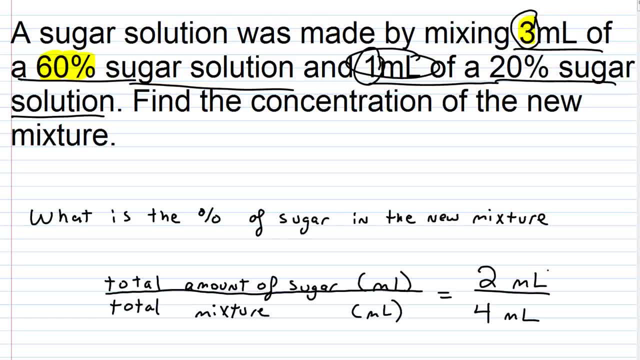 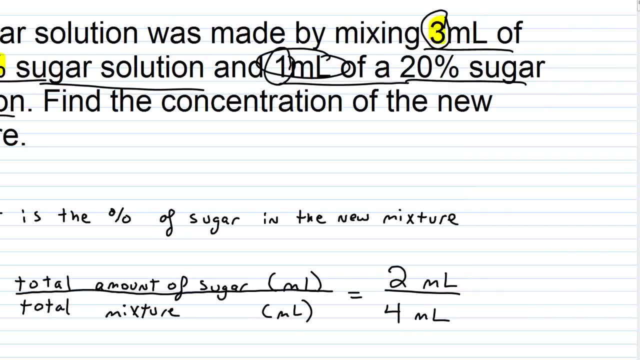 So that's the total amount of sugar in milliliters that's in the new mixture, And then we divide that by the total mixture itself. So we basically have 2 divided by 4, and that's going to be 1, half or 0.5 in decimal form, right. 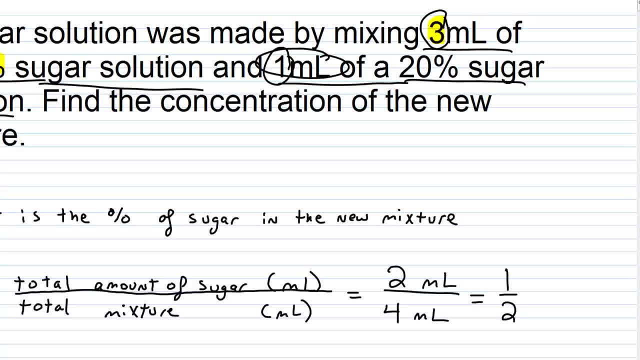 And since we want to write this as a percent, we really want a decimal here, So I'm going to put 0.5. Now as a percentage. 0.5 is going to be 50%. So if I want to write this as a nice little sentence, I go back up here and say: 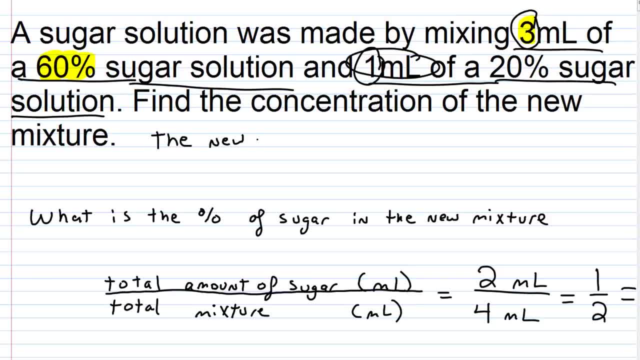 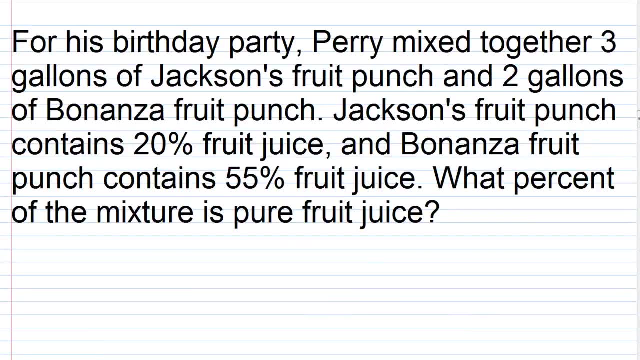 the new mixture is 50% sugar. Let's take a look at another one. For his birthday party, Perry mixed together 3 gallons of Jackson's Fruit Punch and 2 gallons of Bonanza Fruit Punch. Jackson's Fruit Punch contains 20% fruit juice and Bonanza Fruit Punch contains 55% fruit juice. 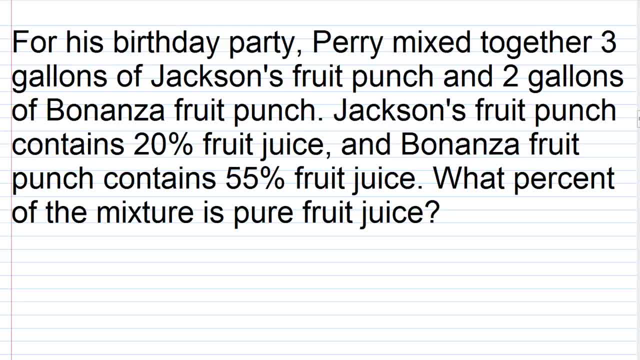 What percent of the mixture is pure fruit juice? So we're basically doing the same thing as in the last problem. Again, I'm going to reread this and I'm going to highlight some important things here. For his birthday party, Perry mixed together 3 gallons of Jackson's Fruit Punch and 2 gallons 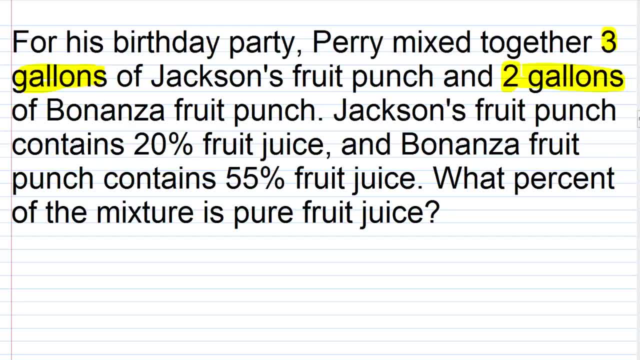 Okay, 2 gallons Of Bonanza Fruit Punch. Jackson's Fruit Punch contains 20% fruit juice and Bonanza Fruit Punch contains 55%. okay, 55% fruit juice. And again the question is: what percent of the mixture is pure fruit juice? 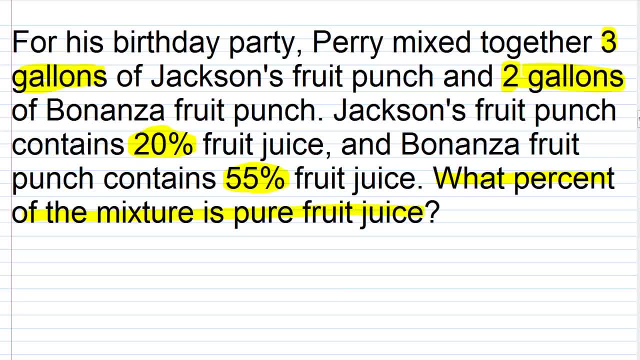 So that's pretty straightforward. So again, we have the same basic formula and what we're going to end up looking for here is the amount of pure, pure fruit juice over the amount of total juice. okay, and this is in gallons and I'm just going to put G-A-L, okay. 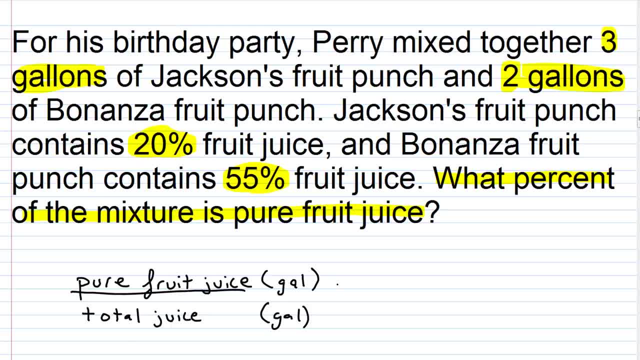 So what would the amount of total juice be? Let's start with that, because that's easier. Well, again, he mixes together 3 gallons of Jackson's Fruit Punch and 2 gallons of Bonanza Fruit Punch. so 3 gallons plus 2 gallons would be 5 gallons. so 5 gallons. 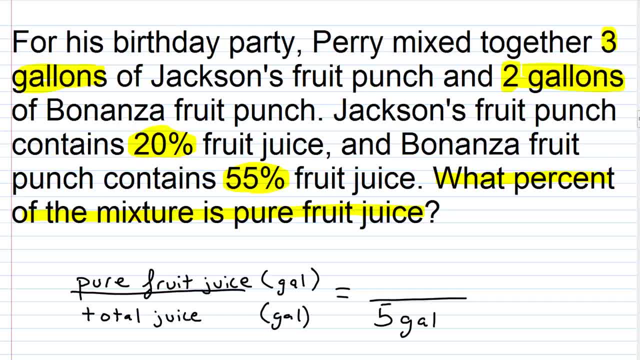 Now how much pure fruit juice is in the mixture? Well, now we've got to do the same thing we did before and take the 3 gallons and figure out. okay, well, out of this 3 gallons of Jackson's Fruit Punch, how much is that as pure fruit juice? Well, we're told 20%. Okay, so we're going to take the 3 gallons and we're going to put G-A-L. okay, well, out of this, 3 gallons of Jackson's Fruit Punch. how much is that as pure fruit juice? We're told 20%. 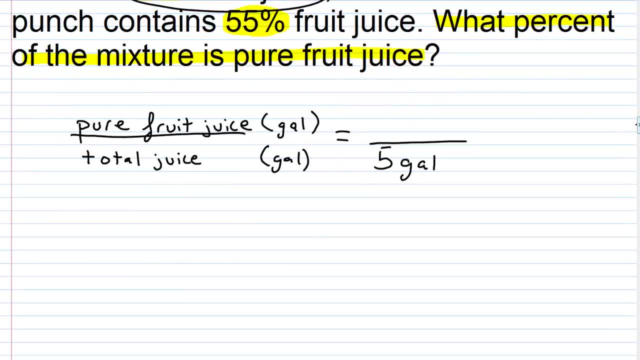 Okay, so we're going to take the 3 gallons and we're going to put G-A-L. okay, well, out of this, 3 gallons of Jackson's Fruit Punch. So what's? 20% of 3 gallons or 20% of 3?? 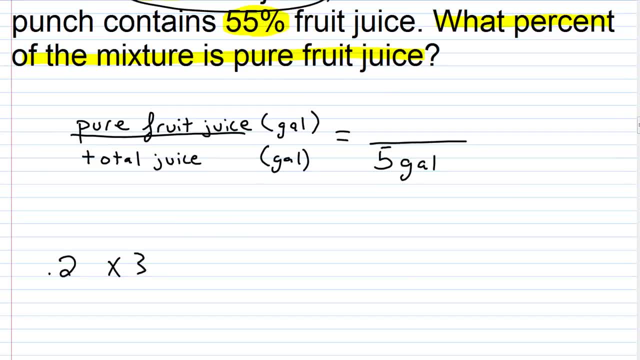 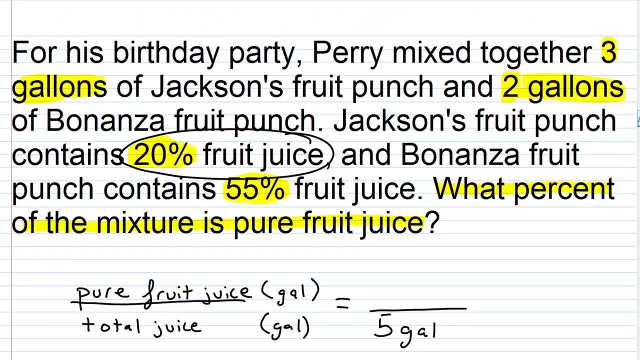 That's 0.2 times 3,, which is going to be 0.6.. Then we need to do the same thing for the Bonanza Fruit Punch. okay, That's 55% fruit juice. so that's 2 gallons. 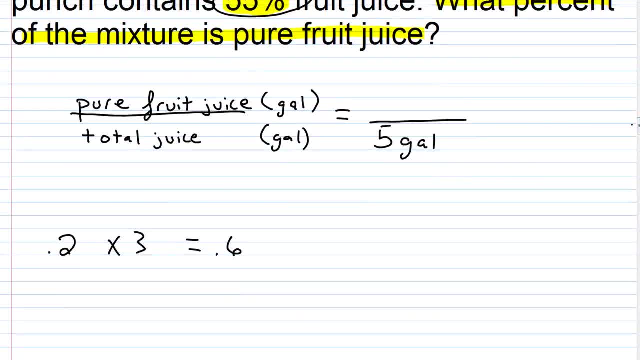 We want 55% of 2 gallons. so 55% or 0.55 times 2.. That's going to end up giving us 1.5.. Okay, so now what we want to do to get the total amount of pure fruit juice right here is: just add these two amounts together, right. 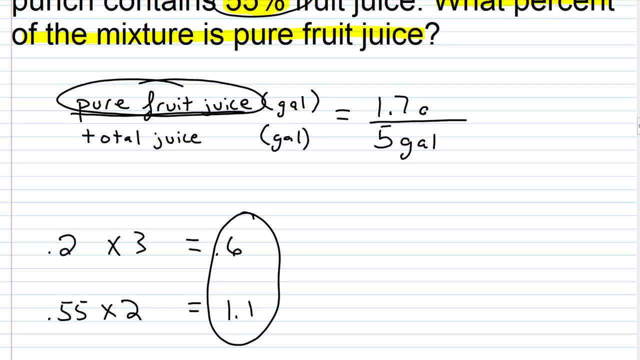 So that would end up being 1.7,. okay, So you have 1.7 gallons of pure fruit juice in this mixture and the total amount of the mixture is 5 gallons. So basically, what we do now is just divide 1.7 by 5..